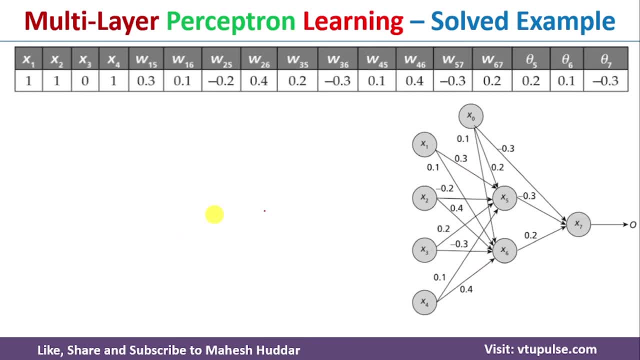 multi-layer perceptron network. Along with this, the weights are also given to us. I have represented that particular weights in this particular table- x1, x2, x3, x4 are the inputs in this case w15, that is nothing but the weight from x1 to x5, which is equivalent to 0.3. 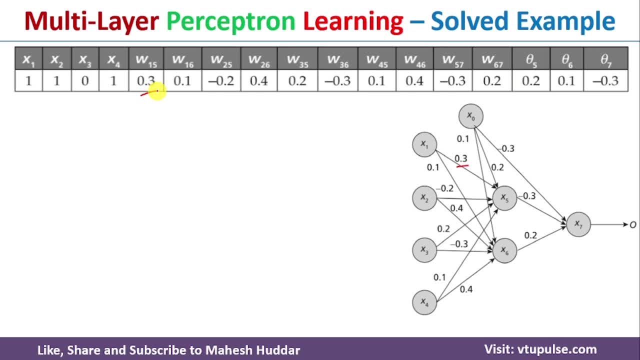 It is given in the network. the same thing I have represented in this particular table w16 is the weight from x1 to x6. here, that is nothing but 0.1. here, the same thing I have written in this case With the same note. I have written all these particular initial weights. 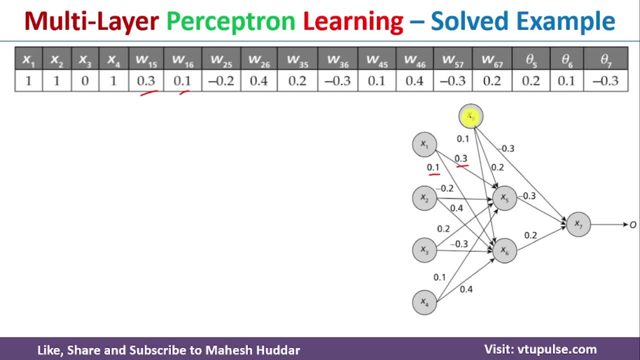 Theta 5 is the weight from this particular bias, that is, x0 to this particular x5, and theta 6 is the weight from x0 to x6. here they are 0.2 and 0.1 respectively, which is also the same thing that I have written here, And theta 7 is the weight from this. 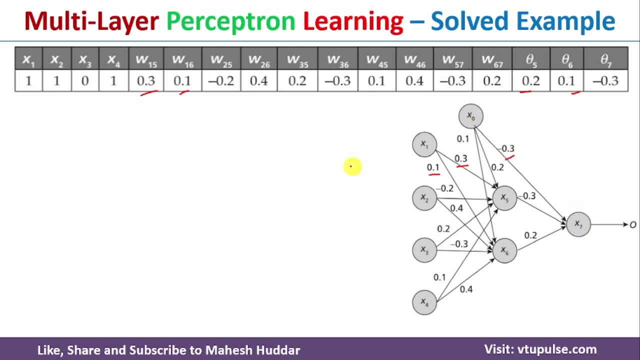 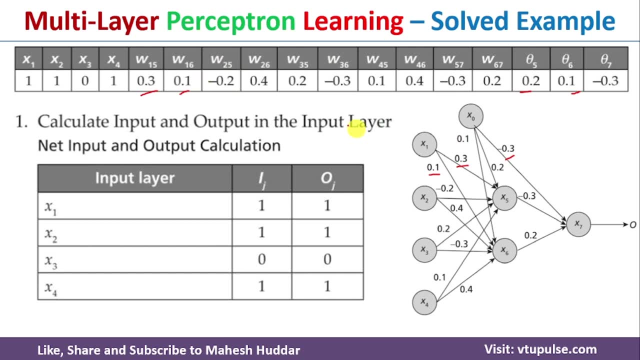 particular bias to this x7, that is equivalent to minus point 3 in this case. haha, here now, given this particular thing, we need to train the multi layer perceptron network and then we need to update these particular weights over here In the first step of multi-layer perceptron. 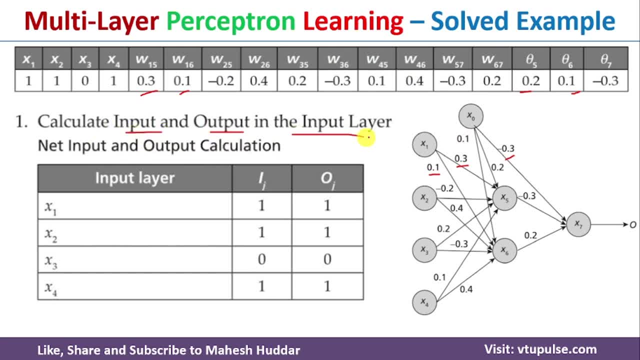 learning. we need to calculate the input and output of this particular input layer neurons. So there are four input layer neurons are there. we need to calculate the input as well as the the input to this particular. x1, x2, x3, x4 are already given to us. the output of this particular. 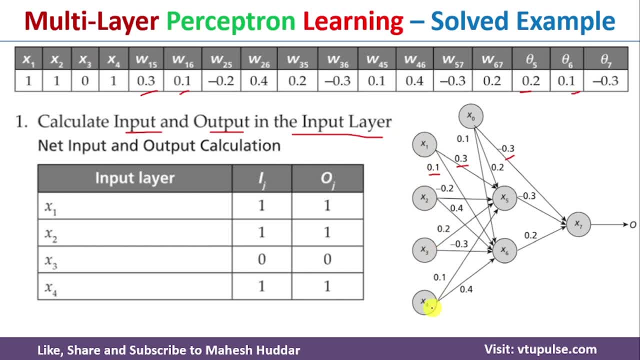 neurons is exactly same because we don't do any modification in this particular input layer. so the output at this particular the input layer neurons is exactly similar to this input. input is 1101 and the output is 1101 respectively over here. so once you calculate the input and 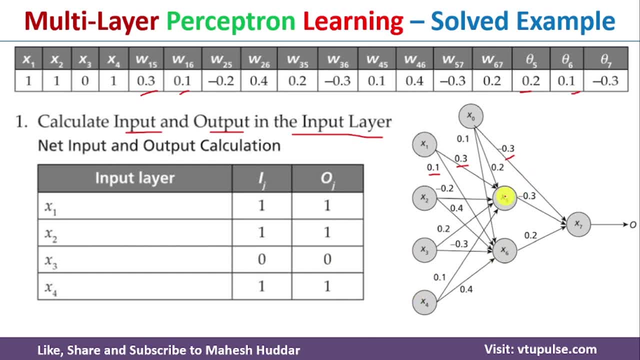 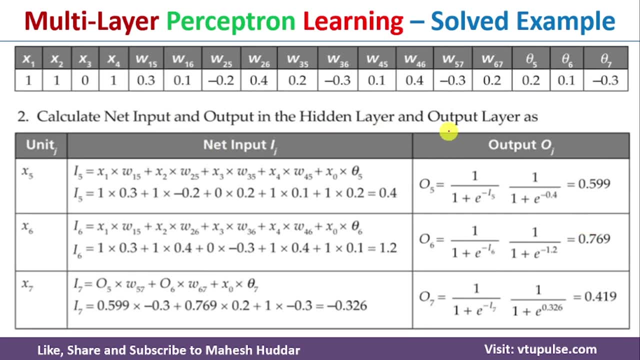 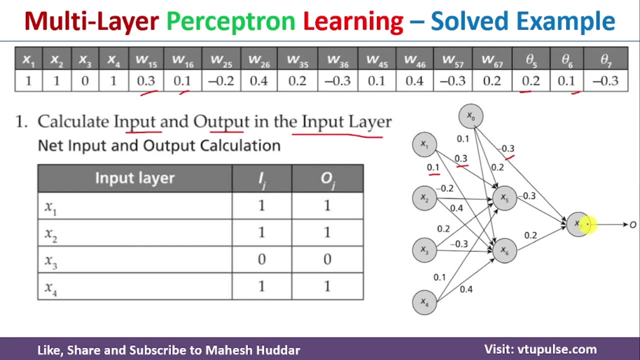 output at this input layer neurons. now we need to calculate the net input and the output at hidden layer neurons as well as the output layer neurons here. so that is what i am doing in this particular table. the hidden layer neurons are x5 and x6 here, and the output layer neuron is x7 in. 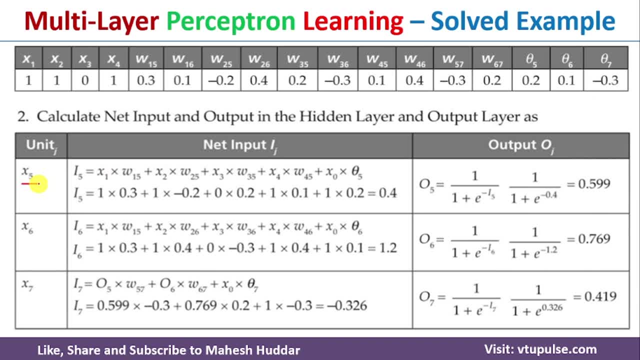 this case. so first we need to calculate the net input for x5 and then we need to calculate the output. here now the question is how to calculate the net input. net input is nothing, but in this case you can see, here i want to calculate the net input at x5. here that is nothing, but we need to multiply the. 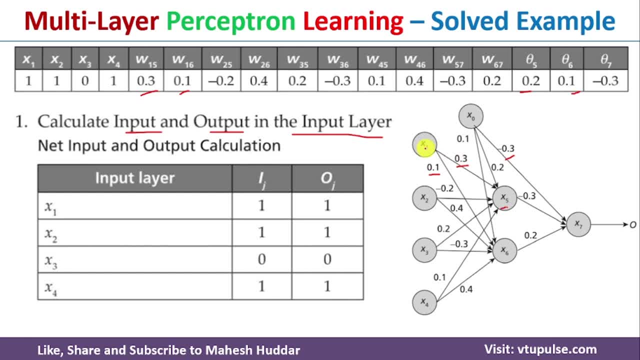 input and the weights over here. so input is x1 multiplied by w15 here, plus x2, w25, x3, w35 and x4 w45 here along with this. so we need to add the bias and its associated weight also, that is x0 multiplied by theta phi here. the same thing i have written in this particular 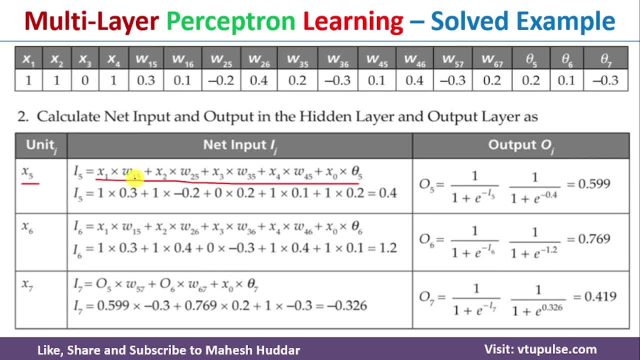 layer here equation that is nothing but x1 multiplied by w15 plus x2 multiplied by w25, and so on. we know the values of all these particular variables. we need to put it over here. you will be getting the net input. in this case, the net input at this x5 is equivalent to 0.4. here, once you get the net input, 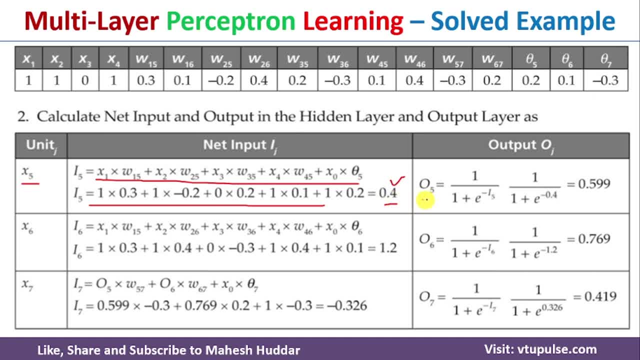 we need to calculate the output at this particular neuron, that is, o5 is equivalent to 1 divided by 1 plus e raise to minus the net input here. so what is the net input? we have calculated? that is 0.4. so 1 divided by 1 plus e raise to minus 0.4. once you solve it, you will get 0.599 in this case. 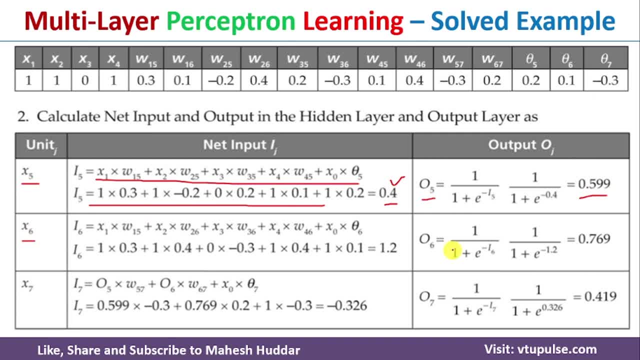 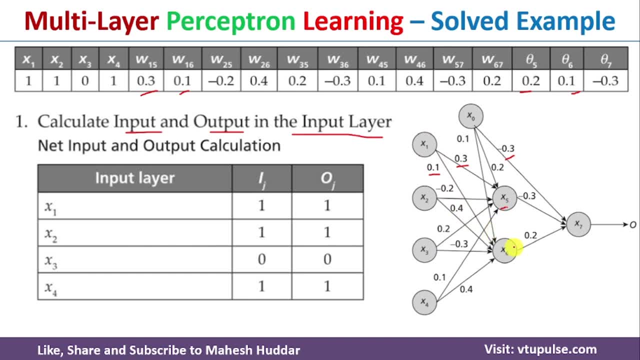 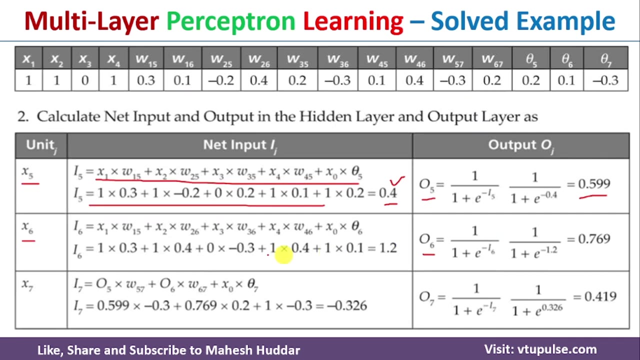 similarly, we need to calculate the net input at x6 as well as we need to calculate the output here. the net input at this particular x6 is x1 multiplied by wx16 plus x2 multiplied by w26, x3 multiplied by w36, x4 multiplied by w46 plus x0 multiplied by theta6. here. that is what i have. 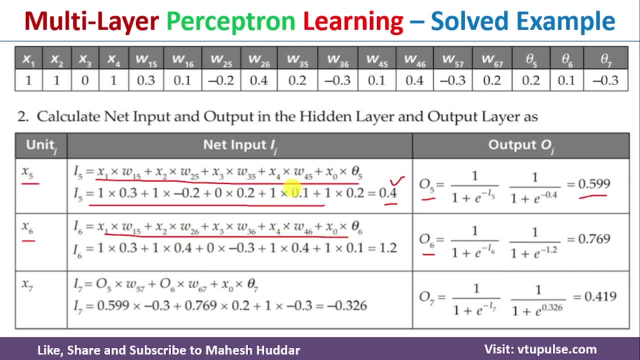 written in this particular equation and then we need to put the values from this particular table. you will get the net input at. x6 is equivalent to 1.2 here and the associated output, that is o6, is equivalent to 1 divided by 1. plus e raise to minus i6. i6 value is known to us, that is 1.2. 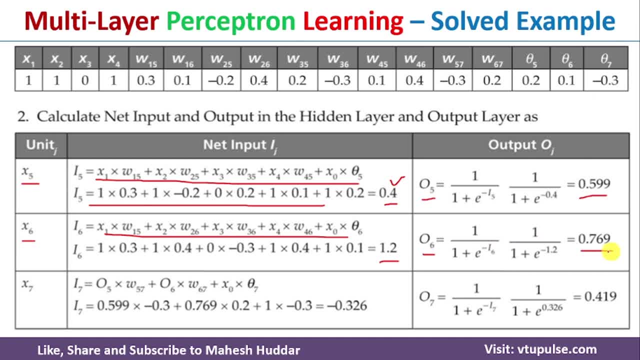 put that particular value in this equation, you will get the output as 0.769 in this case. similarly, we need to calculate the net input at x7. x7 is the output layer neuron, and then we need to calculate the output over here, the output output layer net. 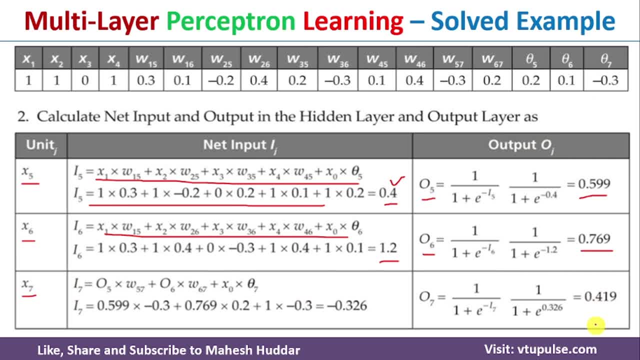 input is calculated here and then the output at the output layer neuron is 0.419 in this case. so this is the output of this particular multi-layer perceptron network in this case. so once you calculate this output at this output layer neuron, we need to calculate the error in. 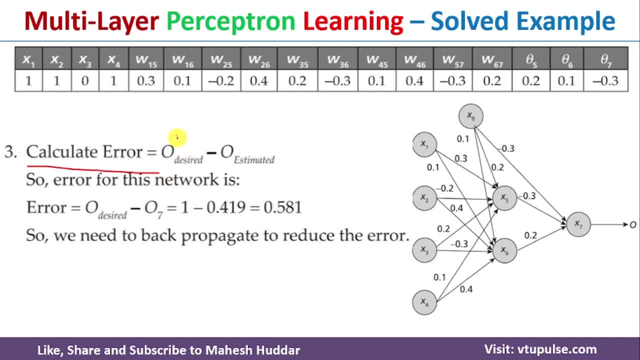 this particular case, the error is always equivalent to o desired. that is nothing but the desired output minus the estimated output. here, what is the desired output? the desired output is equivalent to 1- that is what is given in the problem definition- and the estimated output. that is nothing but the calculated output- is 0.419. that is what we have calculated. 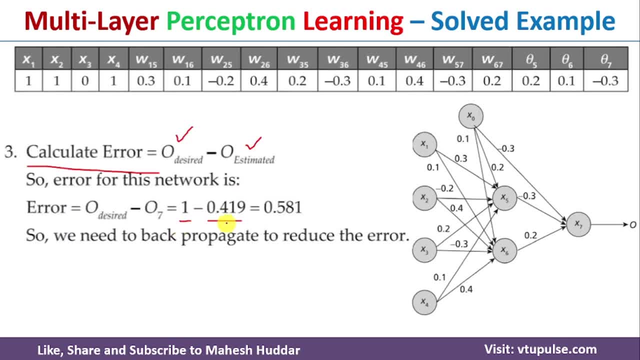 in the previous slide over here. now, once you put these particular values in this equation, you will get the error at the output layer is 0.581 in this case. This is the error, what we got after the first epoch, or you can say that the first iteration. 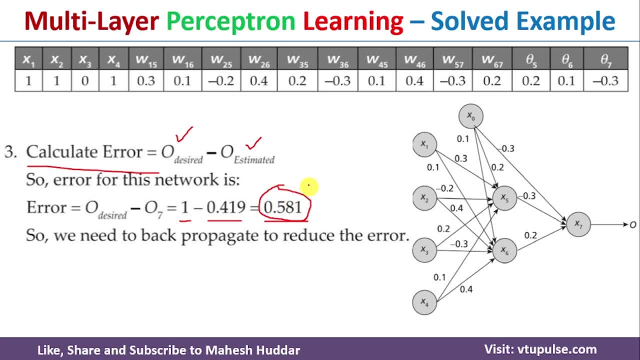 in this case. Now the question is: if you are happy with this particular error, there is no need to do anything here. You can stop the training of this particular multi-layer perceptron network and then you can deploy it in the real world. 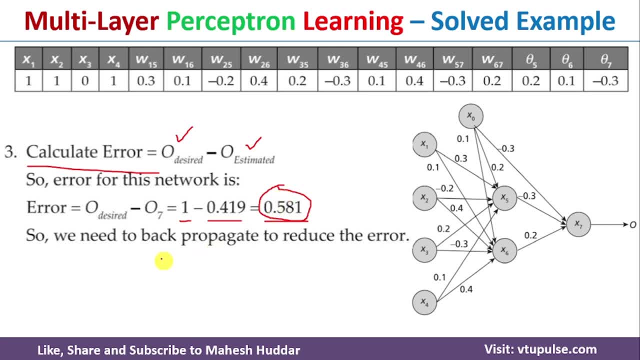 But if you are not happy with this particular error term, what we need to do is we need to propagate this particular error backwards and then we need to update the weights so that we can reduce this particular errors here. So we have been given the weights. 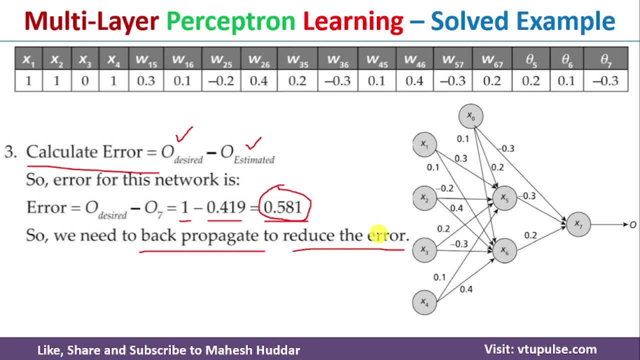 We need to update this particular weights so that we can reduce this particular error in this case. So what we do is we will try to propagate this particular error backwards and then we will try to update the weights and then we will try to see whether the error is reduced. 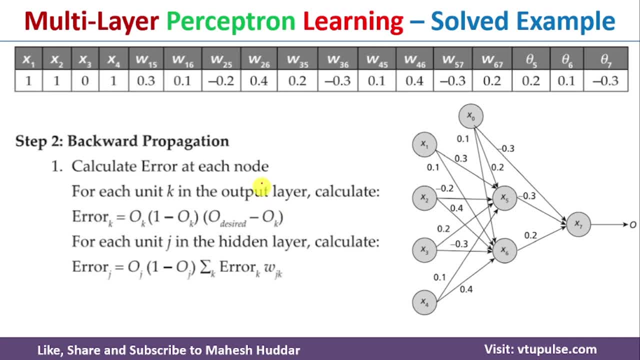 or not in the next iteration, The question comes in point of us is: how can we propagate this particular error backwards? Now, if you want to propagate this particular error backwards, you need to remember these two equations. The one is the error at output layer neurons. 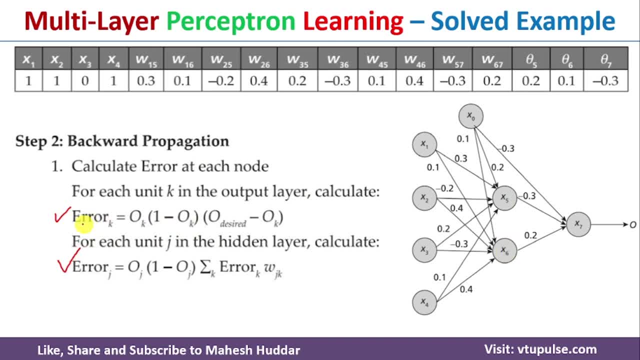 And the error at This particular, the hidden layer neurons. here The error at output layer neuron is always calculated with this equation: OK, that is the output at output layer neuron multiplied by 1 minus OK, multiplied by O. desired that. 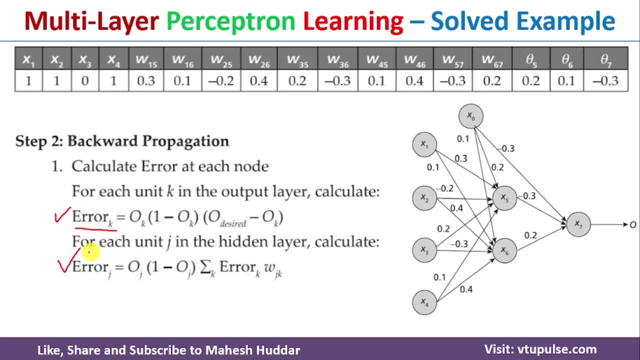 is the desired output minus OK here. And hidden layer neurons. error can be calculated with this equation, that is OJ. OJ is the hidden layer neurons output. 1 minus OJ multiplied by summation of K, K is nothing but what. 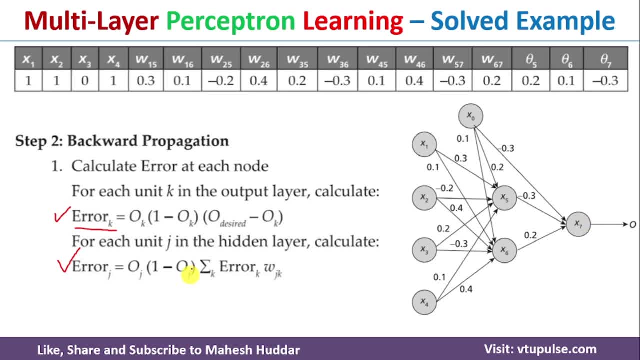 The output layer neurons. In this case we have only 1 output layer neuron. If we have multiple number of output layer neurons, we need to take the summation term over here: Multiplied by error K, That is error at the output layer neuron, multiplied by weight JK. 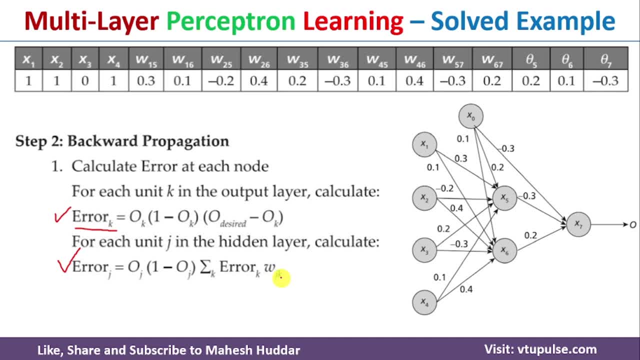 J is nothing but what Hidden layer neuron. K is the output layer neuron in this case. So with this particular equation, we will be able to calculate the error at this particular hidden layer neurons. Once you calculate this particular error, we need to update the weights over here. 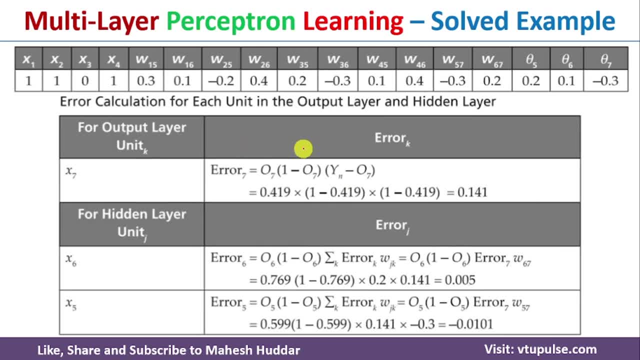 So first we will try to calculate the error at each neuron, OK, neuron. in this case The output layer neuron is x7. For this particular x7, the error is error 7, which is equivalent to o7 multiplied by 1 minus o7 multiplied by yn. that is the desired output. 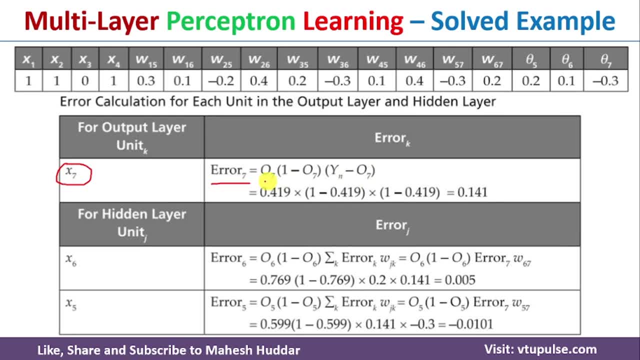 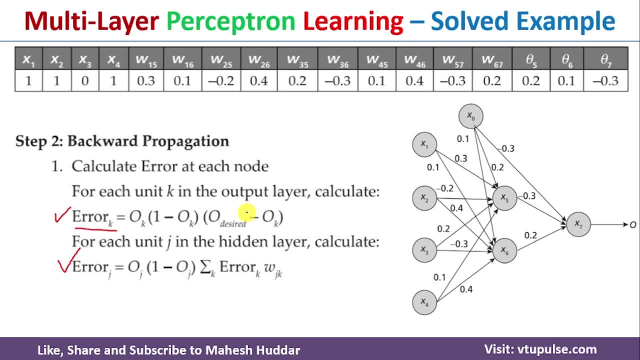 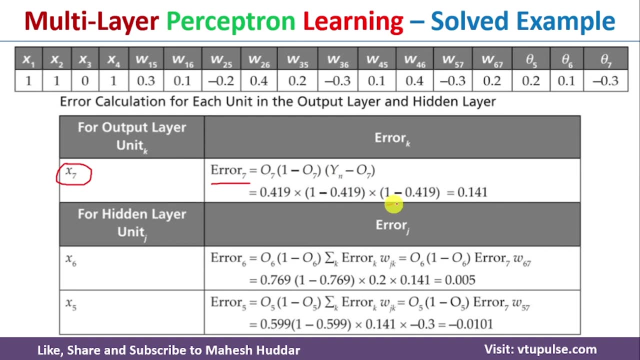 minus the calculated output, that is o7 here. So o7 we have already calculated in the previous slide. that is equivalent to 0.419. that is the calculated output multiplied by 1 minus calculated output multiplied by yn. that is, the desired output is 1 here. The calculated output is 0.419 in this. 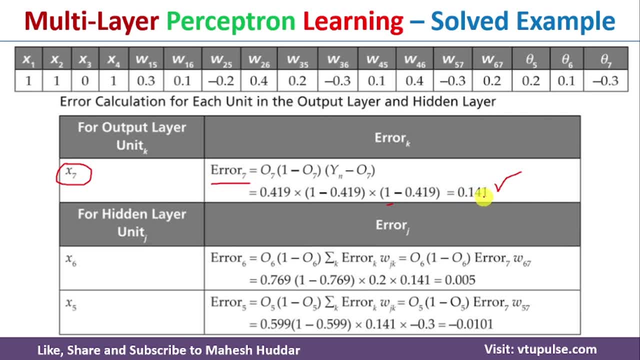 case, and once you solve it, you will get 0.141 in this case. So this is the error term at the output layer neuron in this case. Similarly, we will try to calculate the error at the hidden layer neurons, that is, x6 and x5.. x6 is equivalent to error 6, which is equivalent to o6 multiplied. 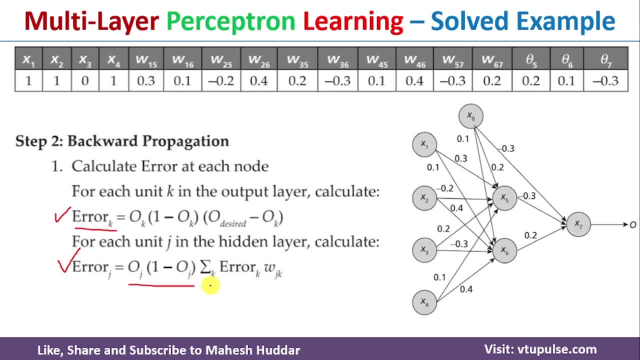 by 1 minus o6- that is what we have written in this case- multiplied by this summation 2.. In this case we have only one output layer neuron, So k will be only once. here This particular summation will not come into picture, because if you have more than one neuron, 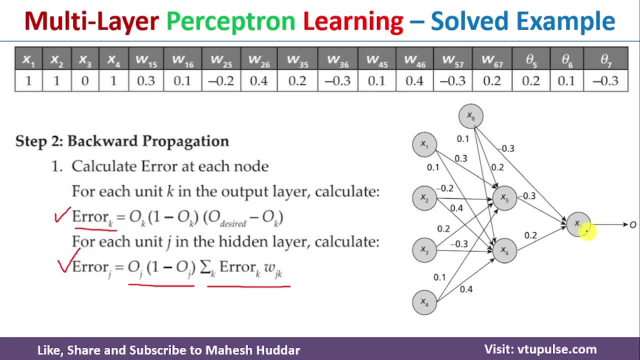 the summation will come into picture. So k value is what, in this case 7 here. So error k multiplied by wj j may be 5 or 6.. If you are calculating error at x5, it will be 5.. If you 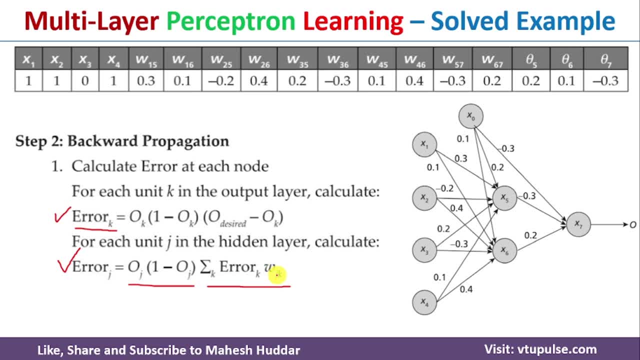 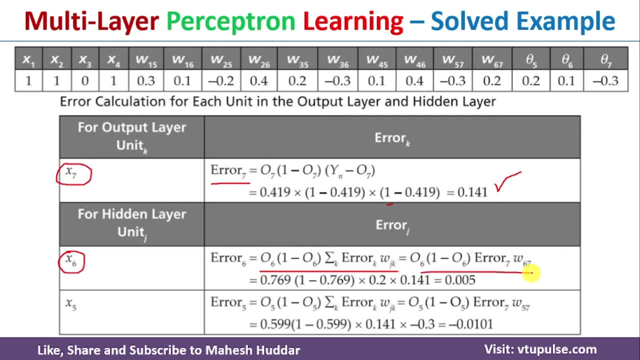 are calculating error at 6, it will be 6 in this case. So w5, w6, k will be 7 in this case. So that is what we have written in this particular equation here, That is, o6 multiplied by 1 minus o6.. Error 7, that is, the 7, is the. 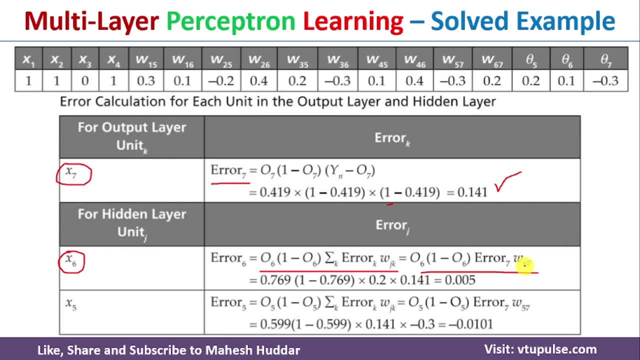 output layer neuron W67,. that is nothing but at 6th neuron. we are calculating the error here. Once you put all the values, you will get this as the error term in this case. Similarly, we need to calculate the error at the 5th layer, 5th neuron. that is equivalent to: 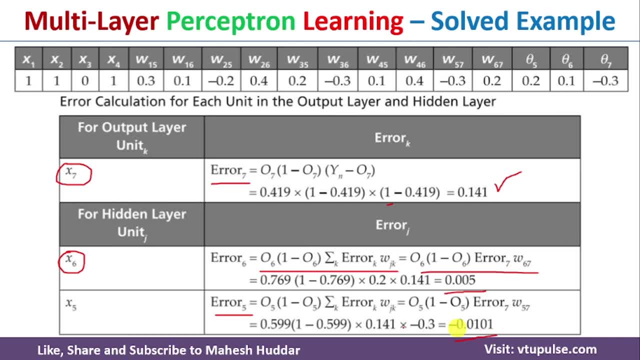 minus 0.0101 in this case. So we have calculated the error at the output layer neuron. We have calculated the error at the hidden layer neurons in this case. Now, once you do this particular thing, we need to update the weights. To update the weights, we need to know the learning rate. 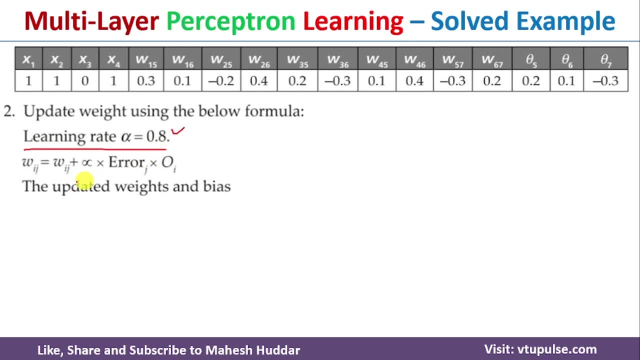 Learning rate is already given to us. that is equivalent to 0.8, as well as we need to know the equation to update the weights. That is, wij is equivalent to wij. that is the old weight plus alpha. that is nothing but learning rate multiplied by error at that particular neuron. 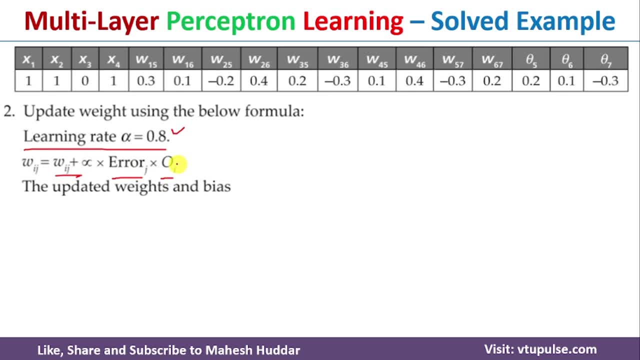 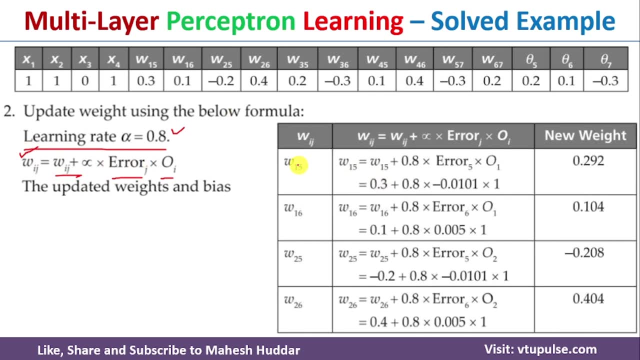 multiplied by the output at that particular neuron here. So once you solve this particular equation, you are going to get the updated weights over here. I will show you few calculations. the remaining you can do it by yourself. W15, that is, we are trying to modify or update the. 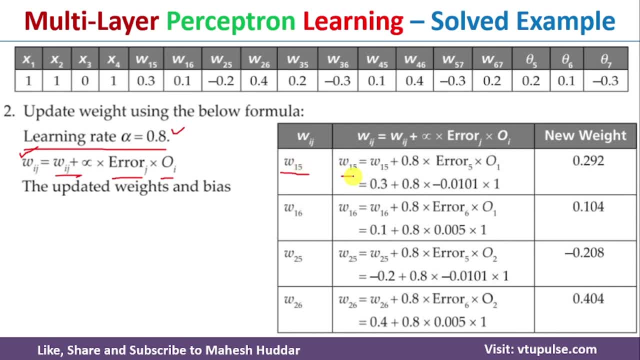 weights at W15 here. So W15 is equivalent to W15, that is the old weight. We know the old weight. What is the old weight over here? That is nothing but 0.3 here plus 0.8.. 0.8 is nothing. 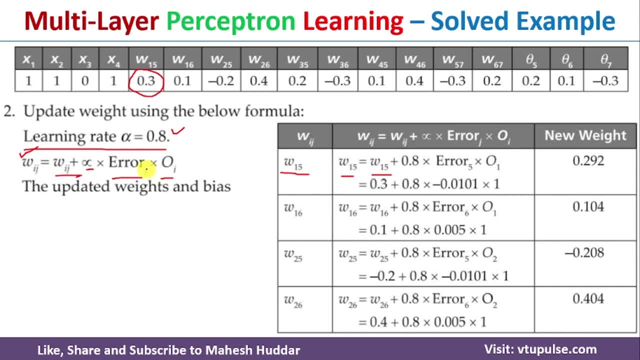 but what Learning rate multiplied by error 5,? that is error 5, we have already calculated in the previous slide. multiplied by OII, I is nothing but what That is in this case. you can see here W15,, that is WIG. So I is equivalent to 1, so that is nothing but O1 here. So O1 is. 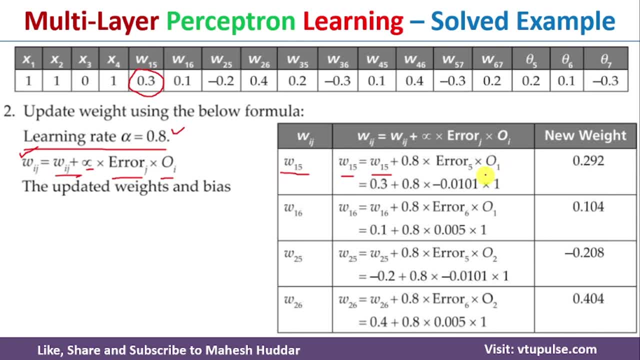 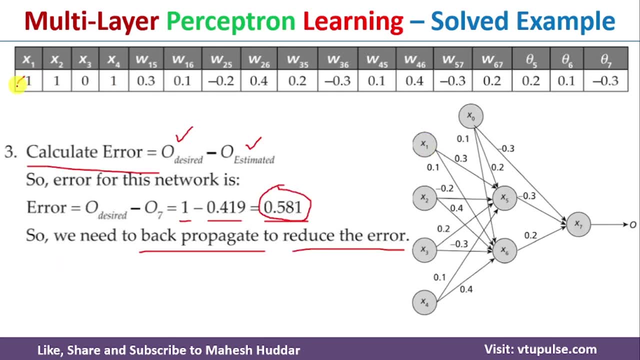 nothing but what: The output at neuron 1, in this case, the output at neuron 1, the neuron 1 is what? in this case, The neuron 1 is. this is X1, the output at this particular neuron is nothing, but the input only. that is nothing but 1 over here. So that is what I have added in this. 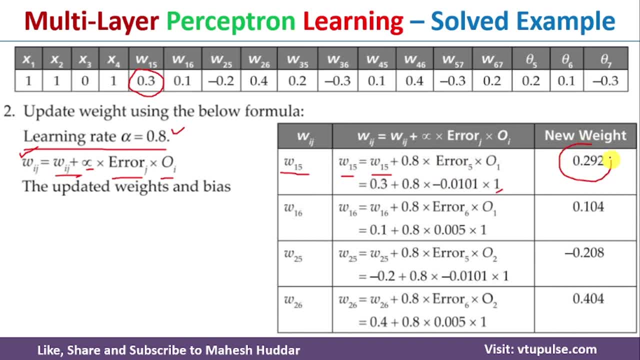 particular case. So once you solve this particular equation, you will get the new weight in this case. Similarly, we need to calculate or update the weights at W16, that is, W25,, 26,, 35,, 36,, 45,, 46 and so on. So the updated weights are written in this particular. 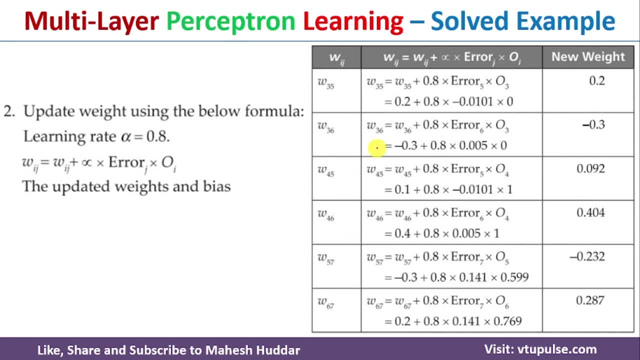 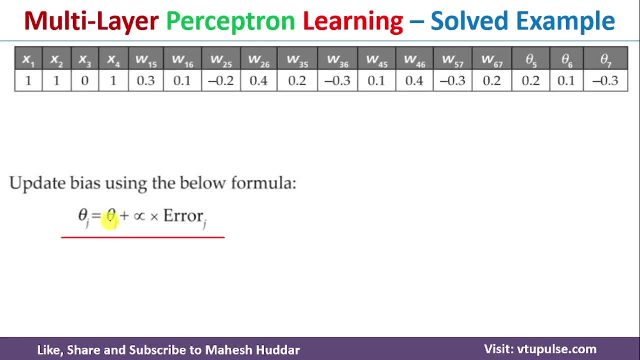 table here. So once you update this particular weights, the next step is to update the bias here. To update the bias, we use this particular equation, that is, theta j is equivalent to theta j plus learning rate multiplied by error. here. We do not consider output here, because output is: 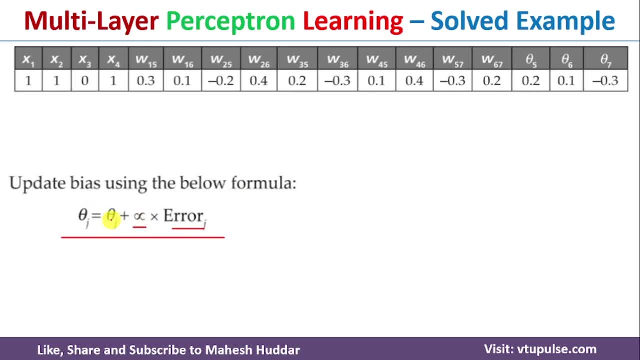 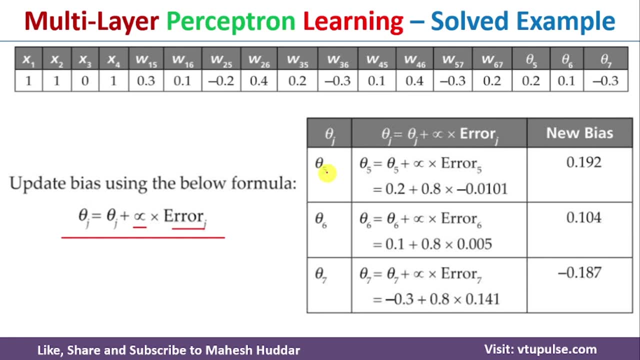 in this particular case. So we do not consider output, only we consider the old weight plus learning rate multiplied by the error at that particular neuron in this case. So theta 5 is equivalent to theta 5 plus theta 5 is the old weight plus alpha. that is nothing but the learning. 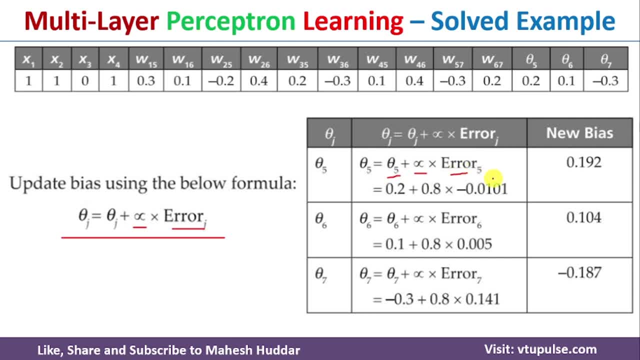 rate that is equivalent to 0.8, error 5.. Error 5 is already known to us. We put all these particular values. we will get the new bias here. Similarly, we need to calculate theta 6 as well as theta 7 in. 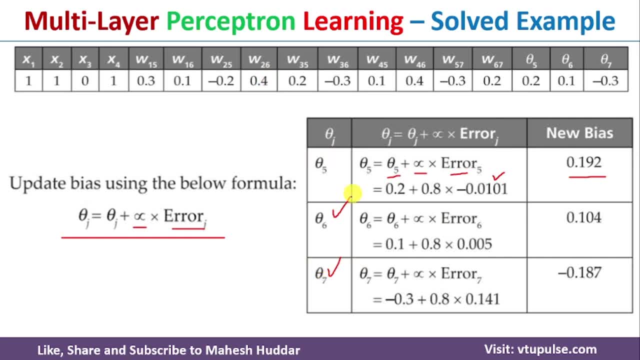 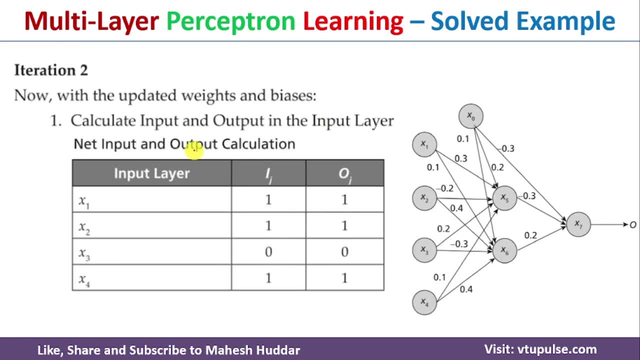 this case. So once you calculate the updated weights as well as the updated biases here, now what we need to do is we need to find the. I can say that we need to propagate the input again from input layer neuron to output layer neuron and then we need to calculate the error over here. So in the first 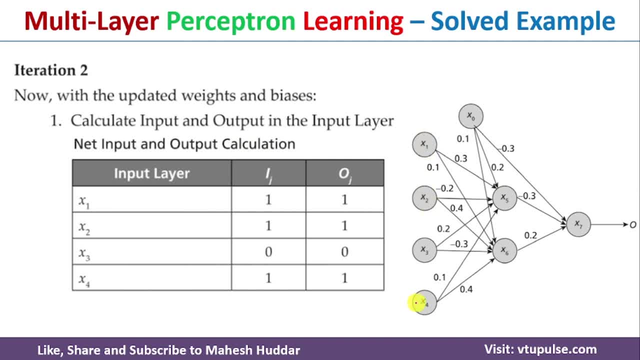 step again, we need to calculate the output at the input layer neuron. The output at input layer neuron is exactly similar to the input here. So input is 1, output is 1 here, input is 1, output is 1 here, and so on. So there is no need to do any calculation at the input layer neuron. 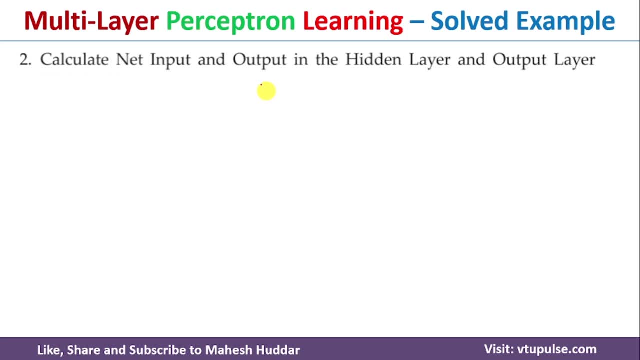 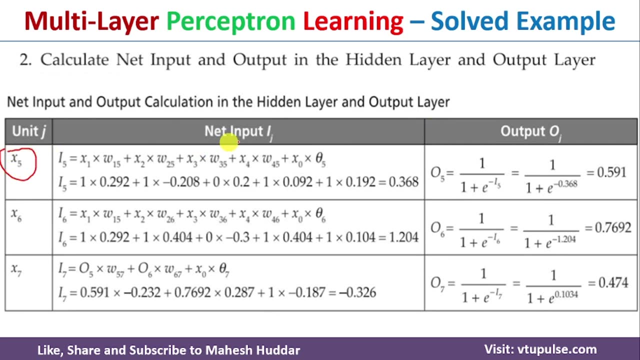 Now we need to calculate the net input as well as the output at the hidden layer neuron as well as the output layer neuron here. So that is nothing but x5, we need for x5, we need to calculate the net input as well as the output over here. This equation I have written already in the previous. 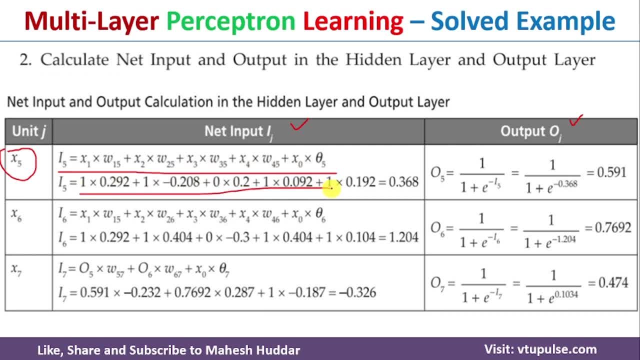